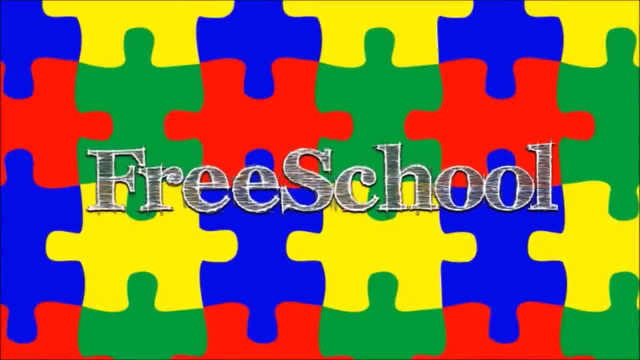 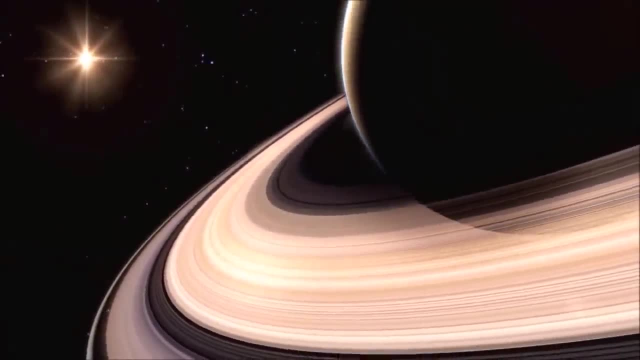 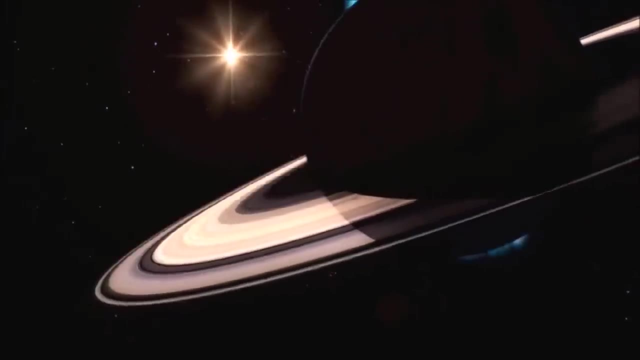 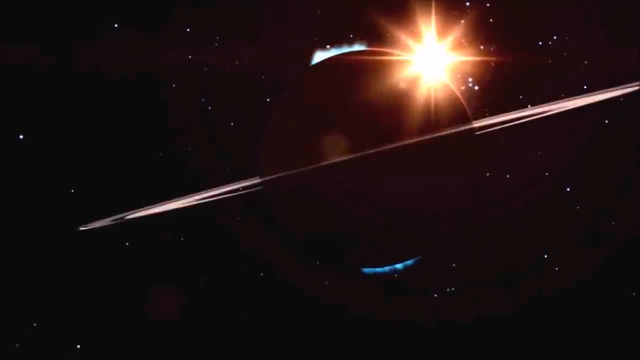 Saturn, the sixth planet from the Sun, is the second largest planet in the Solar System, smaller only than Jupiter. Saturn is easy to identify because of the large, beautiful system of rings surrounding it. Like Jupiter, Uranus and Neptune, Saturn is a gas giant. 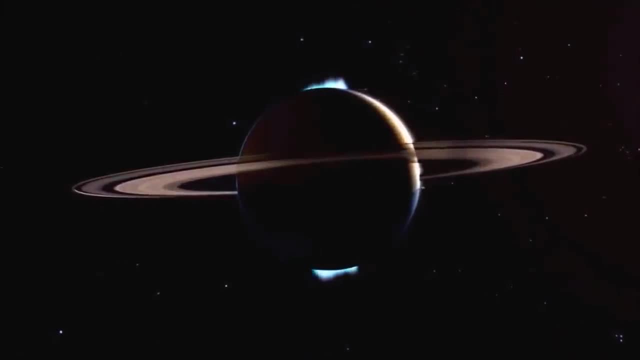 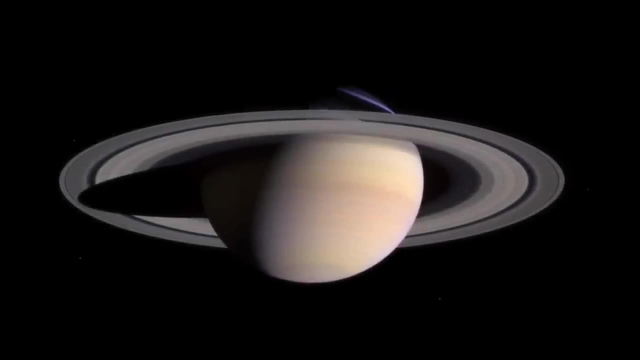 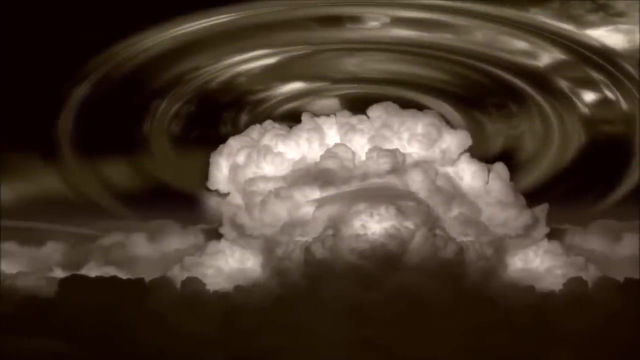 It is made mostly of hydrogen and helium, with crystals of ammonia in the upper layers of its atmosphere, which is what gives it its pale yellow color, Although the outermost layers of Saturn are made of gases. scientists believe that if you traveled down through 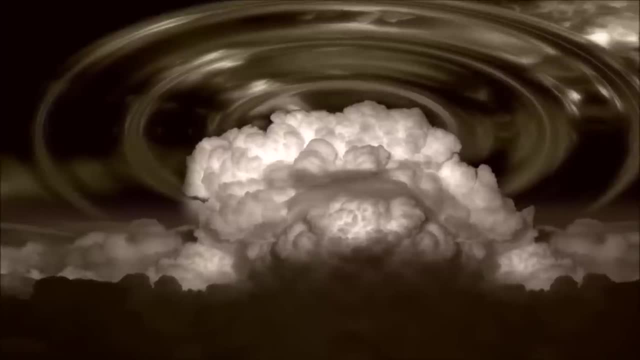 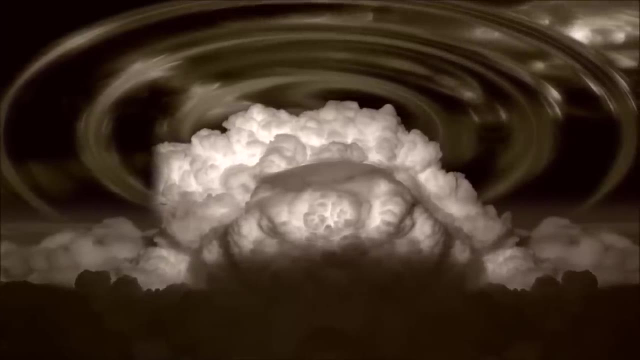 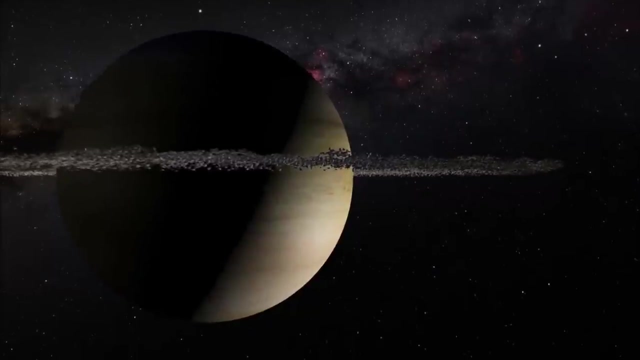 the atmosphere, you would eventually find that the hydrogen and helium became liquid and, even farther down, metallic, and in the center of the planet, they believe, there is a hard rocky core. Saturn is the least dense planet in the Solar System, Although it is much larger than the. 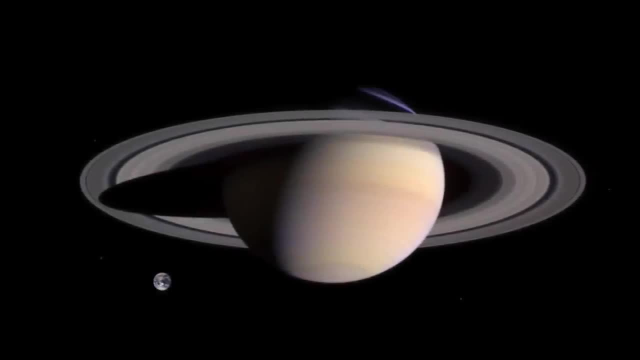 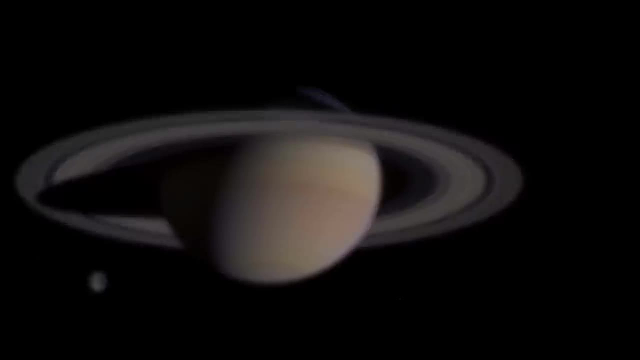 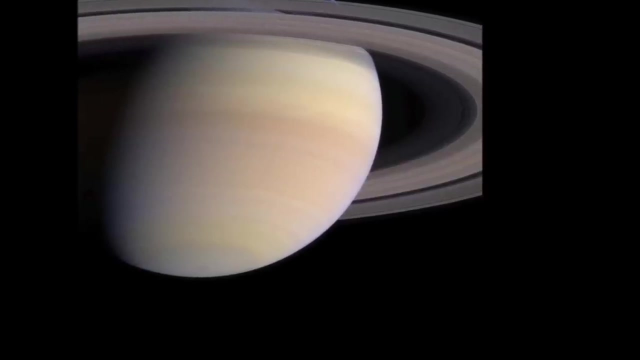 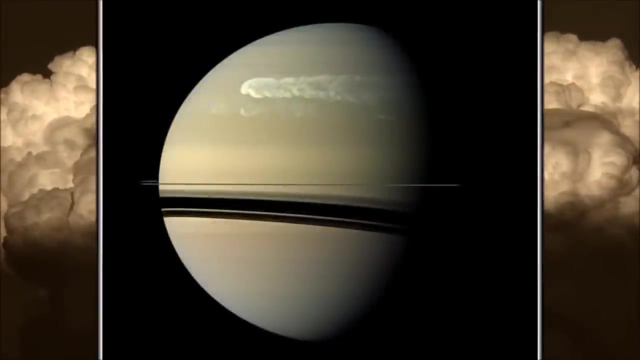 Earth about 9 times wider and 95 times more massive. it is only about 12% as dense as the Earth is. This means that if you were able to find a bathtub large enough, Saturn would float in the water Like Jupiter. Saturn has storms and stripes of clouds. They are just harder to see because 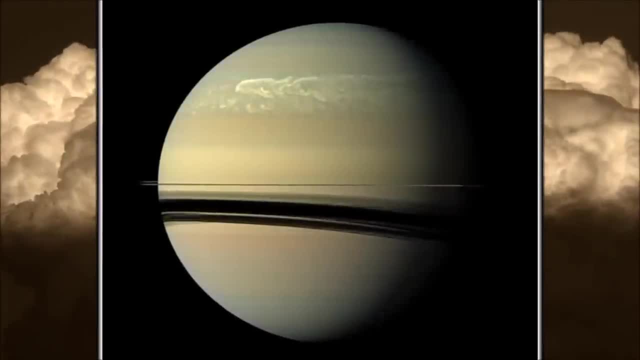 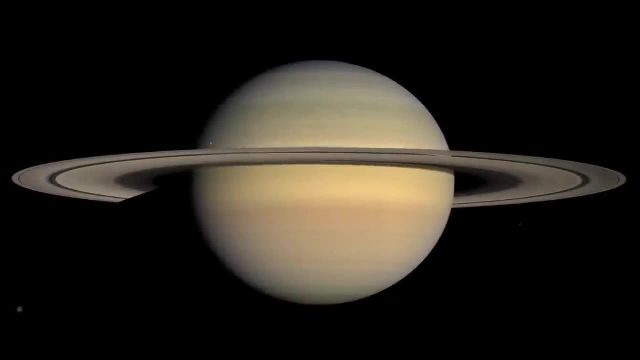 of their pale color. However, winds on Saturn are much faster than Jupiter s winds. Saturn has the second fastest winds in the Solar System, reaching speeds of 1.7 times the speed of the Sun's temperature. That is to say, if you were able to find a bathtub large enough, Saturn would float in. 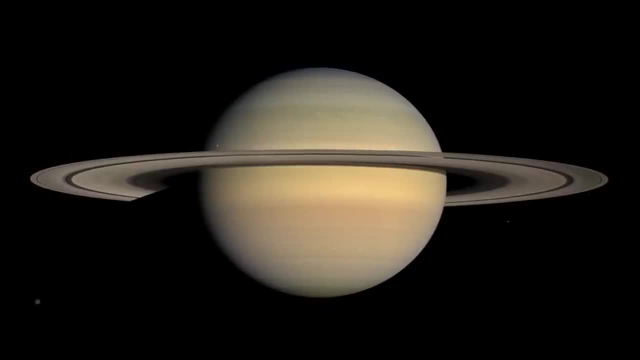 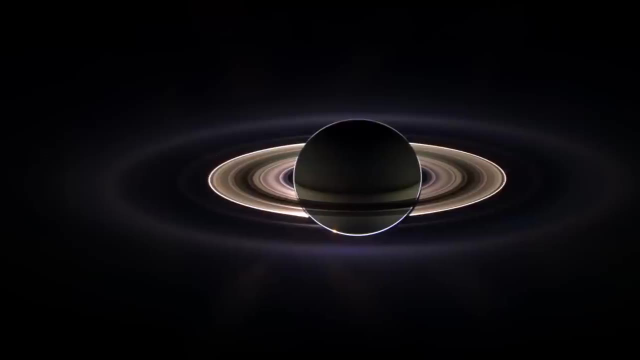 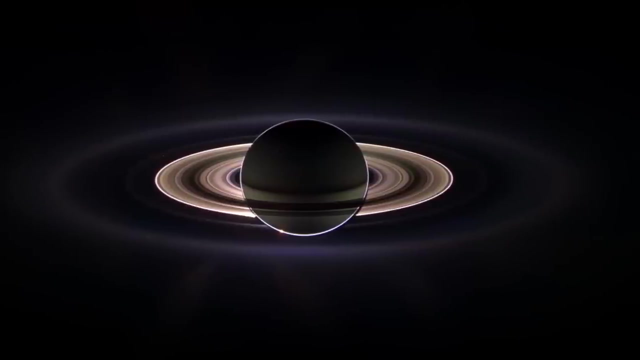 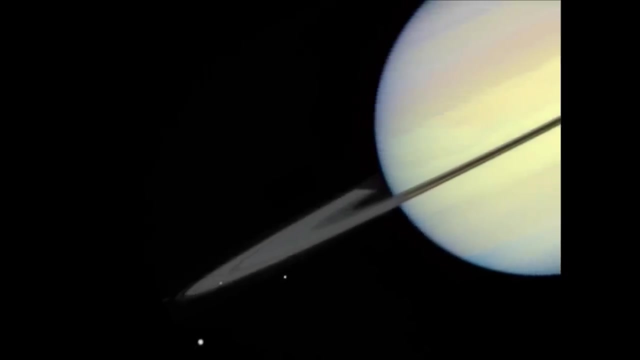 the water, reaching speeds of 1,800 kilometers per hour. The only planet with winds faster than Saturn is Neptune. Saturn is far from the Sun, about 890 million miles or 1.4 billion kilometers away. As a result, it takes a very, very long time to travel around the Sun: about 29 years. 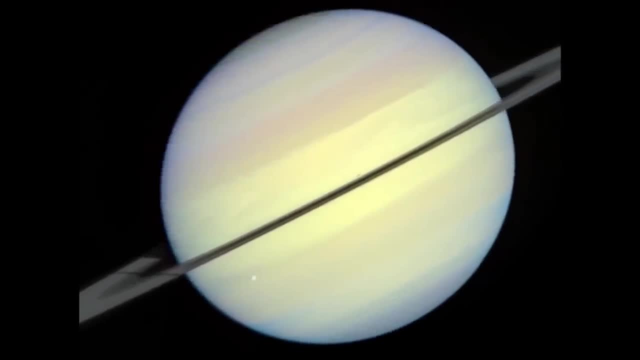 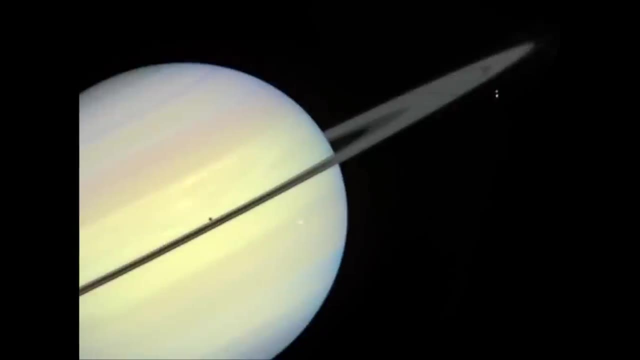 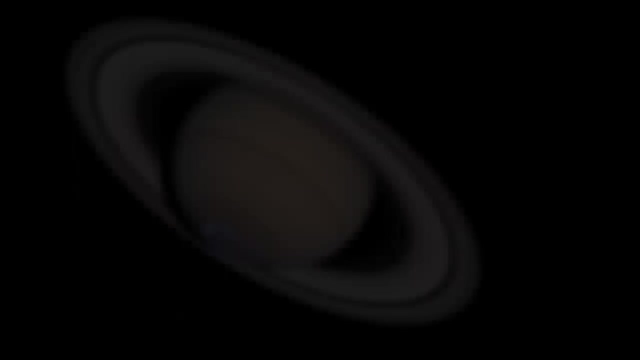 However, it spins or rotates much more quickly than the Earth does. Instead of rotating once every 24 hours, Saturn's day lasts less than 11 hours. Saturn is the farthest planet that can be seen by humans without help from a telescope. 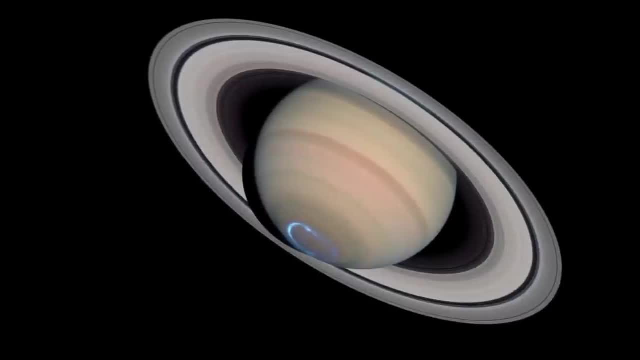 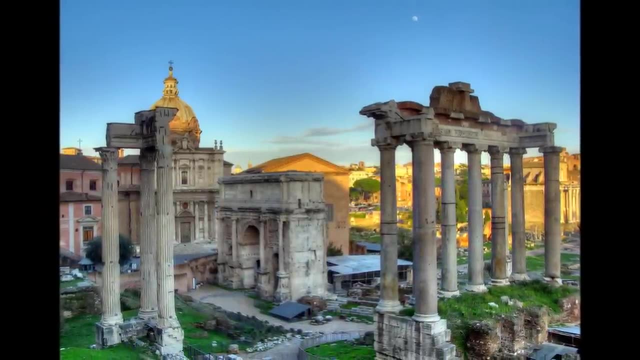 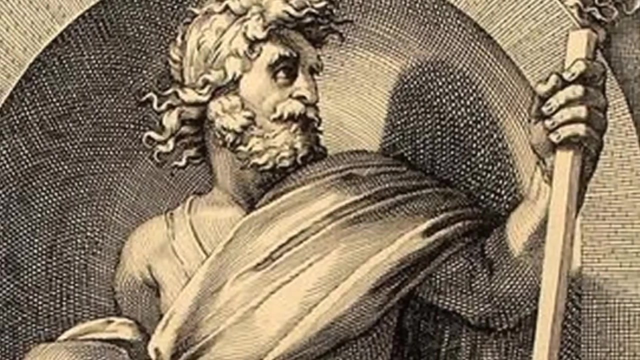 and so it has been known to humans for thousands of years. The ancient Babylonians, Greeks, Romans, Chinese and Japanese astronomers and more all had a name for Saturn. The word Saturn comes from the name of the ancient Roman god, Saturnus, god of wealth. 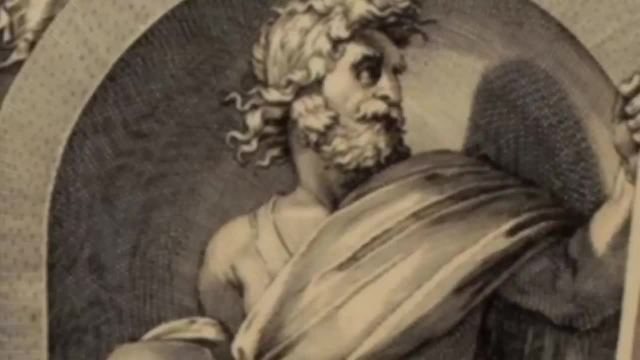 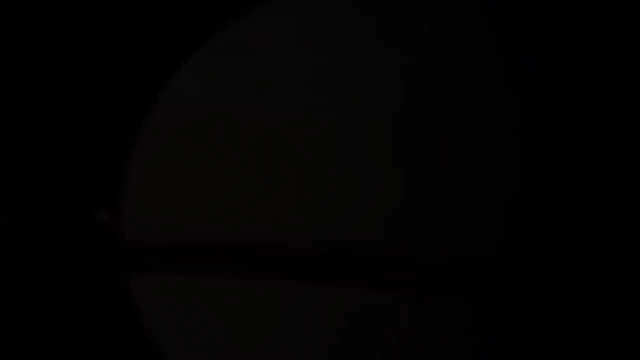 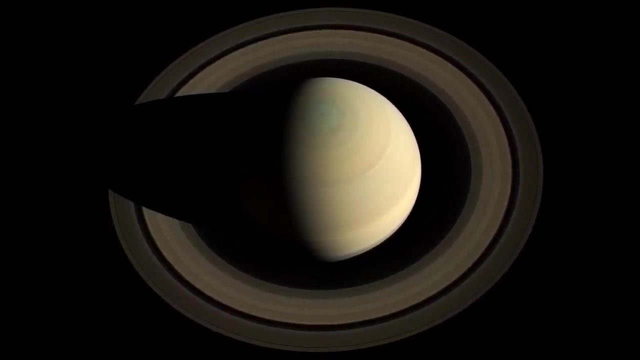 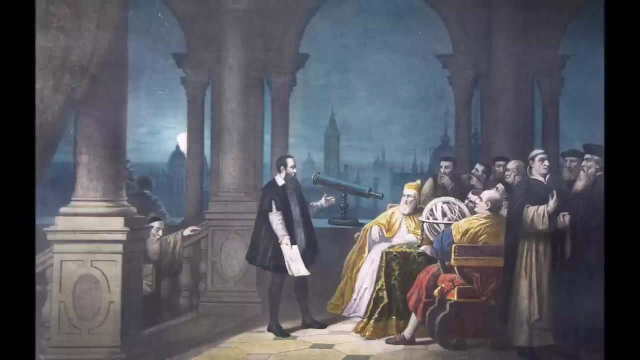 and agriculture. Although ancient astronomers knew about Saturn, no one knew about its rings. The rings are not visible without the help of a telescope, and so it wasn't until the astronomer Galileo used his telescope to observe Saturn in 1610 that people knew that there. 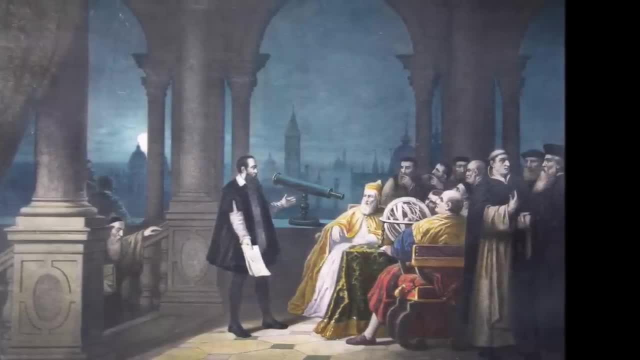 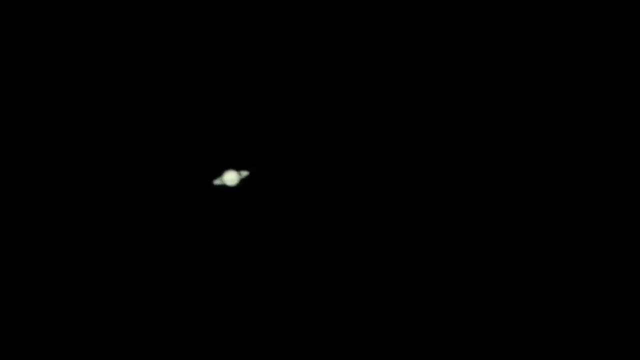 was anything different about it at all. When Galileo saw Saturn's rings, he didn't know what they could be. He thought they might be moons or smaller planets set beside the main one in the center. He even described the rings as the rings of Saturn. 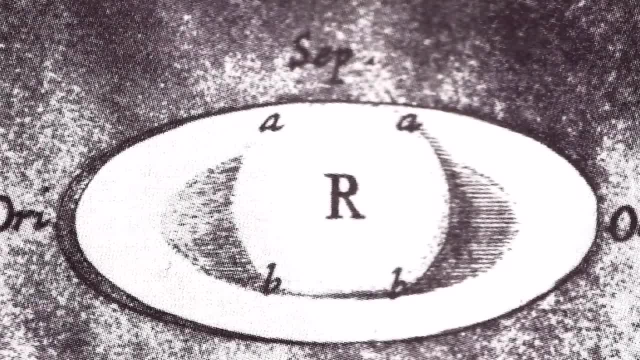 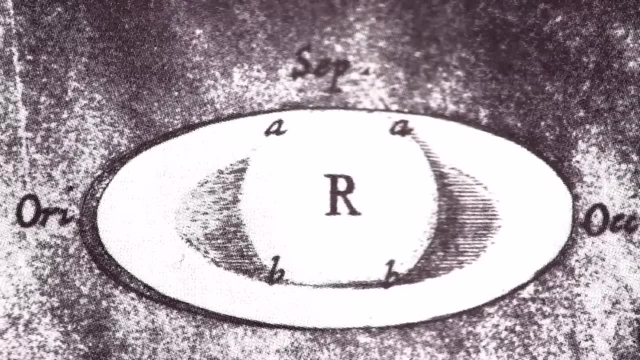 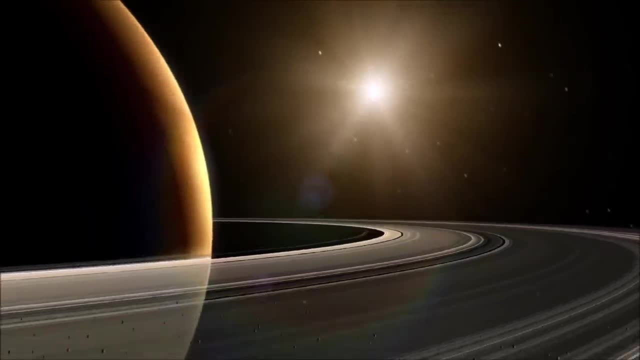 The rings that the Galileo said were the rings of Saturn, Saturn's ears. It wasn't until later, when stronger telescopes were made, that astronomers realized that Saturn was surrounded by wide flat rings. Saturn's rings are about 175,000 miles or 282,000 kilometers across, but only about 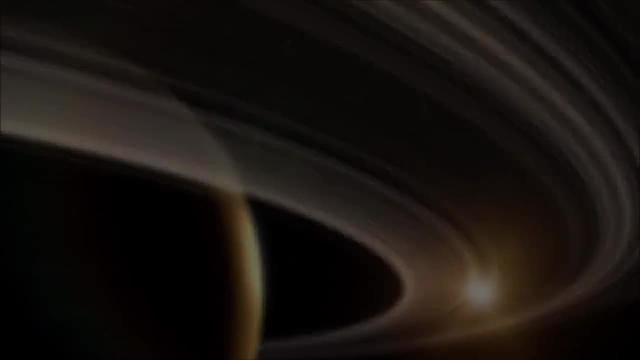 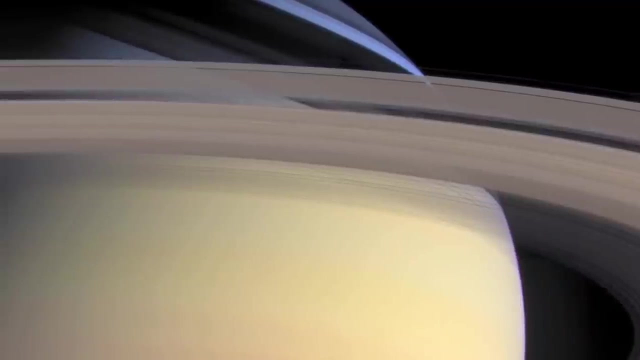 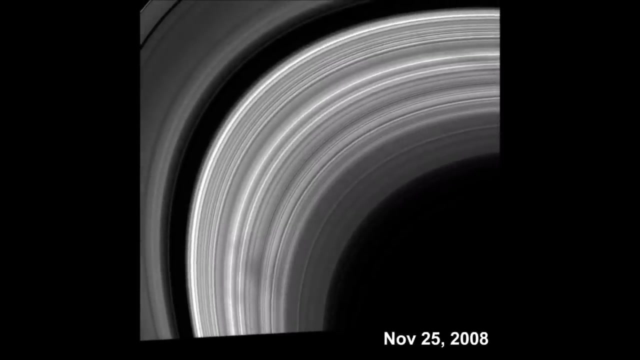 30 feet or 10 meters thick. They are made of many, many pieces of ice and rock, ranging from the size of a grain of sand to the size of a bus. Scientists believe that the rings may have formed when comets, asteroids or even moons.